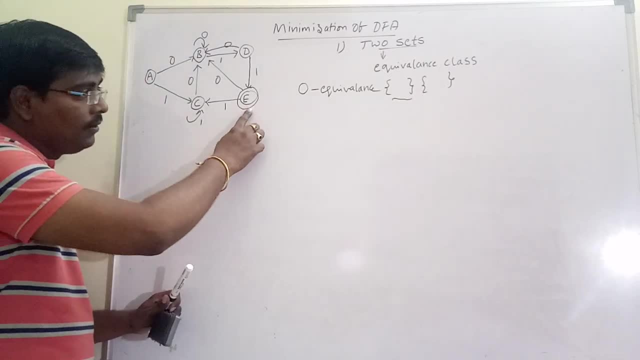 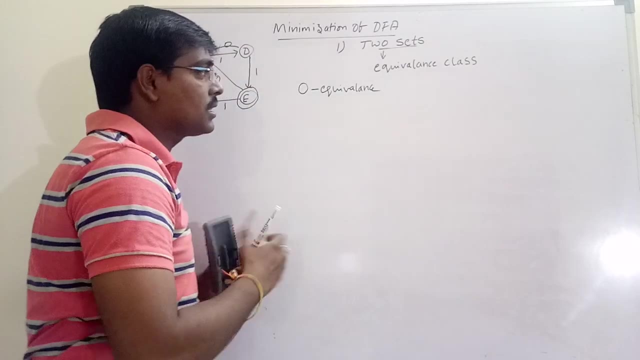 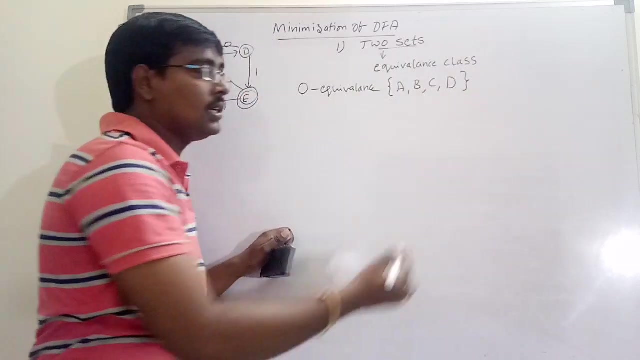 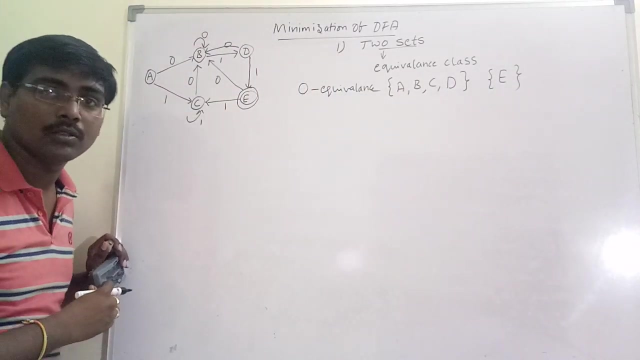 In the given diagram we have only one final state and remaining A, B, C, D are non-final states. So zero equivalence class has two sets: A, B, C, D becomes one set and final state E becomes another set. This is the first way. So the first step is constant zero equivalence class. So I am converting this into: 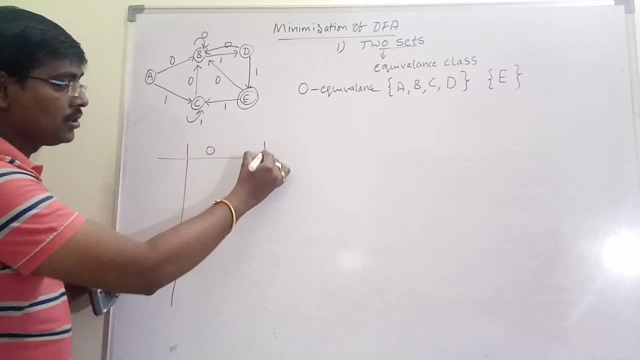 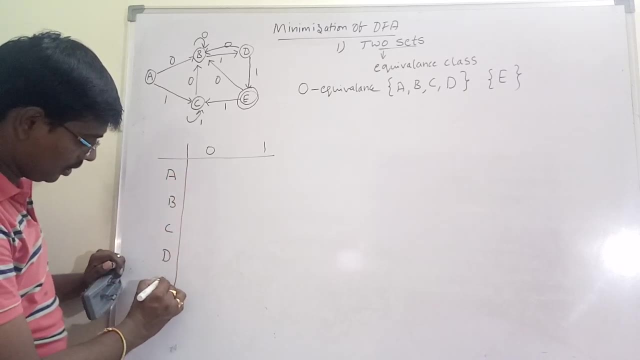 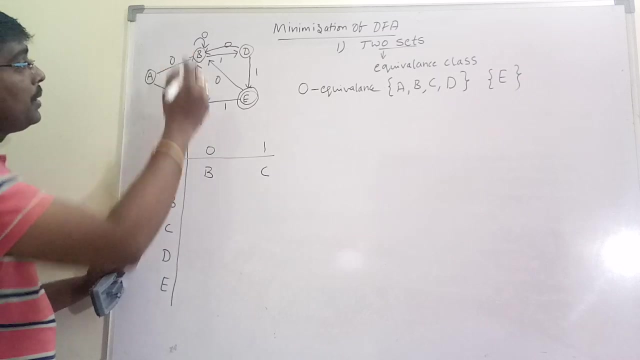 transition table for easy calculations. Inputs are zero and one States are A, B, C, D, E. A on input zero. we are moving to B. A on input one. we are moving to C. Next B on input zero, B, B on input one. we are moving to D. C on input zero, B, C on input one, C. 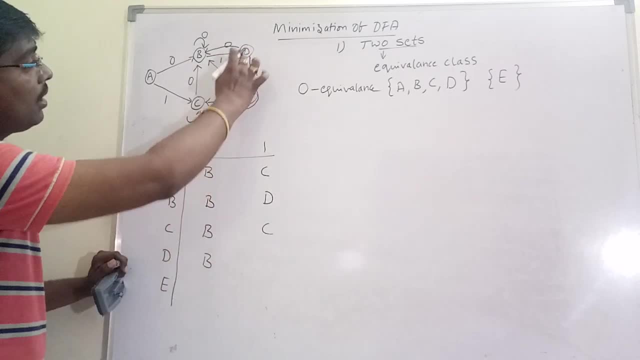 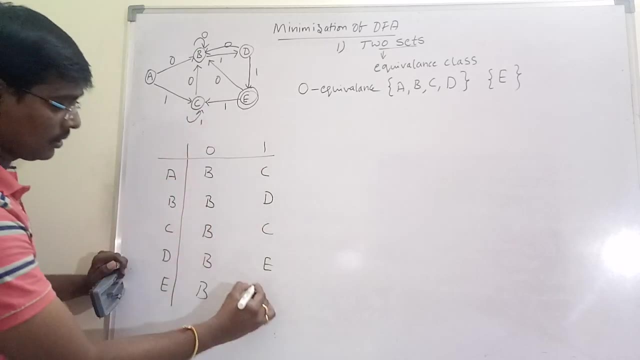 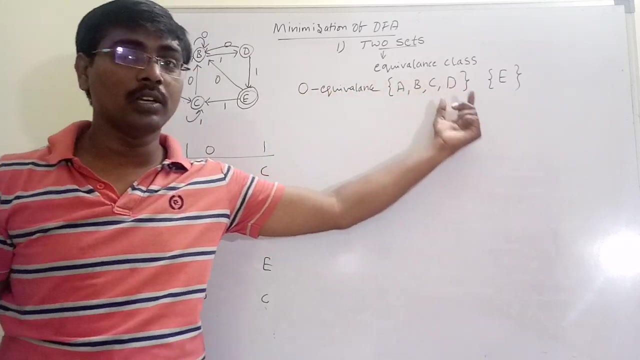 D on input 0, B. D on input 1, E. E on input 0, B. E on input 1, C. This is the translation table And first convert, first construct 0 equivalence class which contains only two sets: One is non-final states and another set is final states. 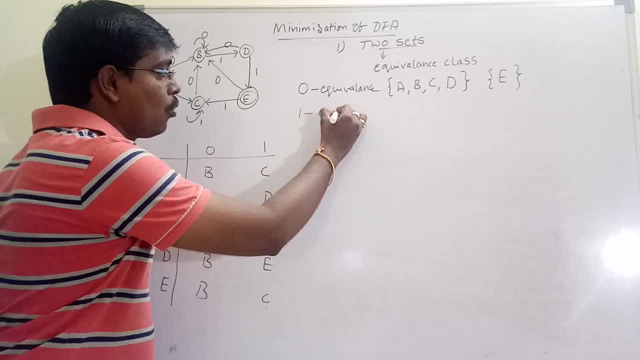 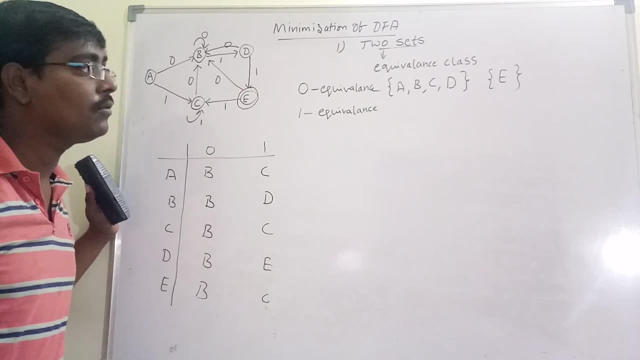 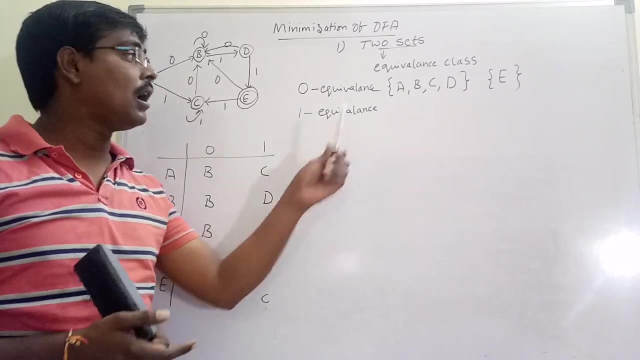 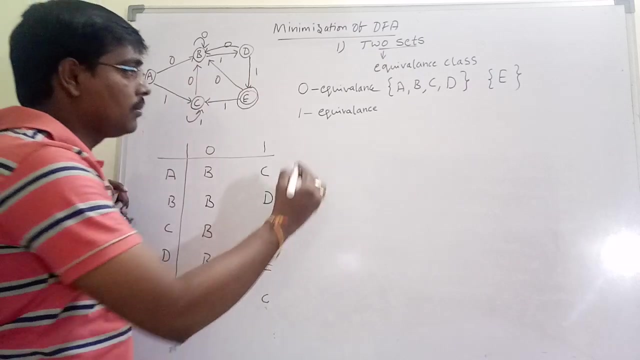 After that we have to find one equivalence class, One equivalence class that is baseline, single input. We are providing the sets into different number of sets, That is, which two states are equivalent on a transition, Suppose on input symbols, which two states moves to the same equivalence class. For example: first you calculate delta of A, 0.. 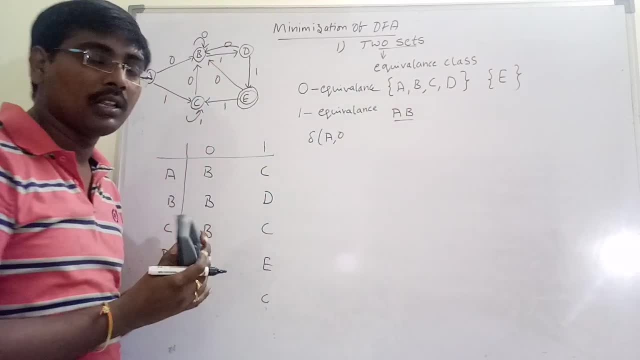 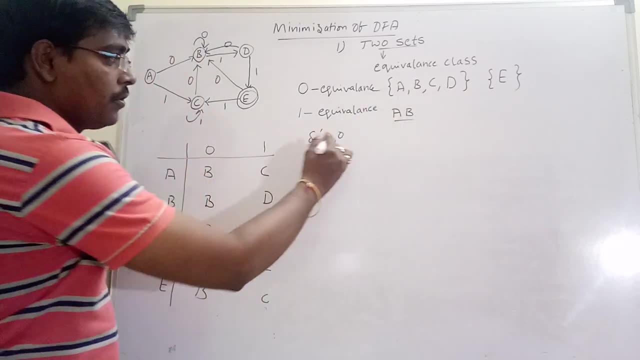 First I want to calculate delta of A- 0.. I want to check A- B Check whether the two states, A and B, are equivalent or not. To check whether two states are equivalent or not, first to perform delta of A- 0.. 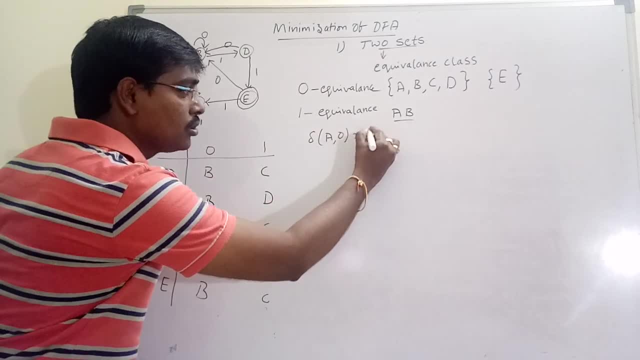 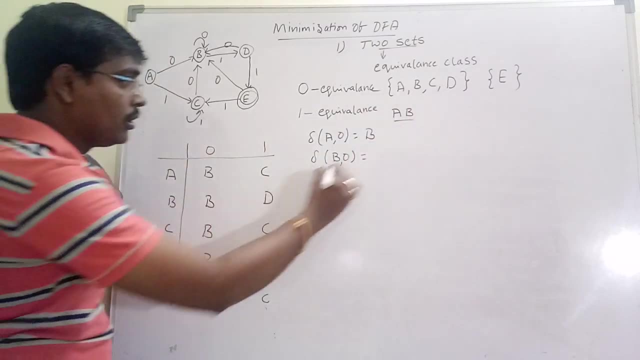 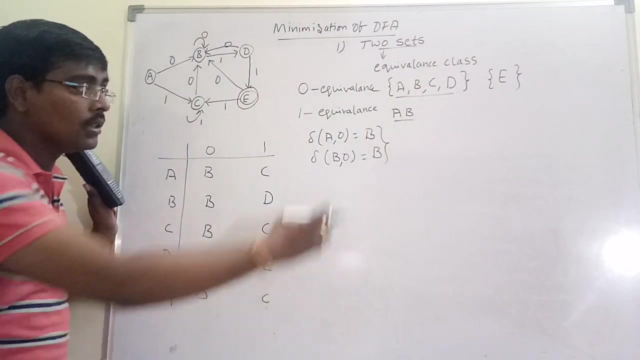 Delta of A on 0, it moves to state B, Delta of B: 0.. So next delta of B: 0, it moves to state D, So these B's belong in a single set. Then after 2 transitions, 2 two-step JK. 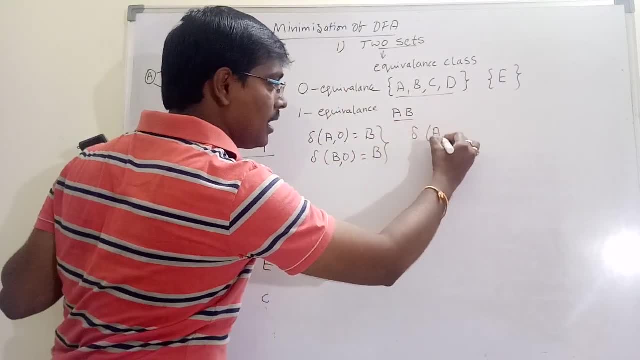 Then let's see which set B is equivalent, for D is a single set. now let's see whether or not these two states Next calculate delta of A- 0, 1 and delta of B- 0, 0.. 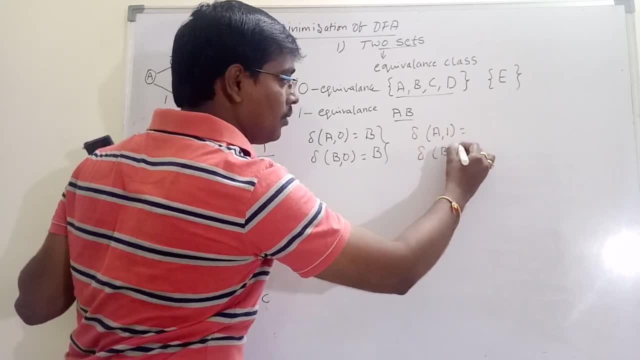 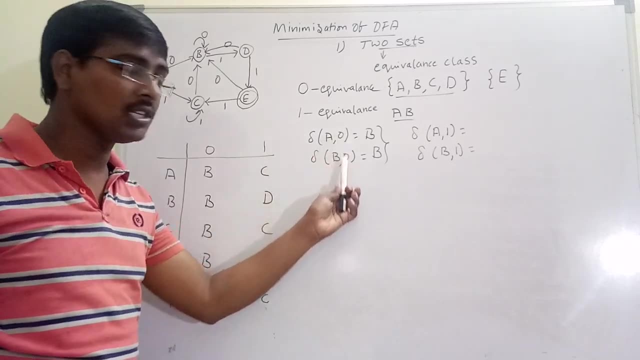 To check whether two states are equivalent or not. Next calculate delta of A, 0,, 1 and delta of B, 0.. For that, in two states, find the transitions with the input symbols. Because if two set are equivalent, then if they move to same setthen, those two sets are equivalent. 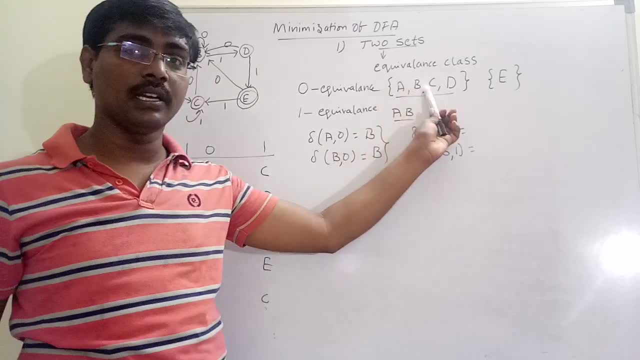 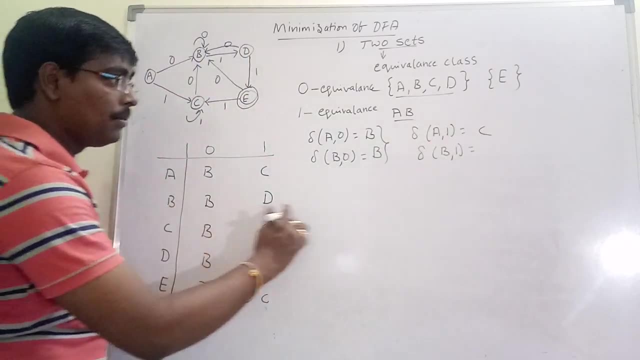 If they move to the same set, then delta of A: 0, 1 is C. Delta of B- 0, 1 is D. Both terms are equivalent to each other. Delta of A: 1 is C: 0.. 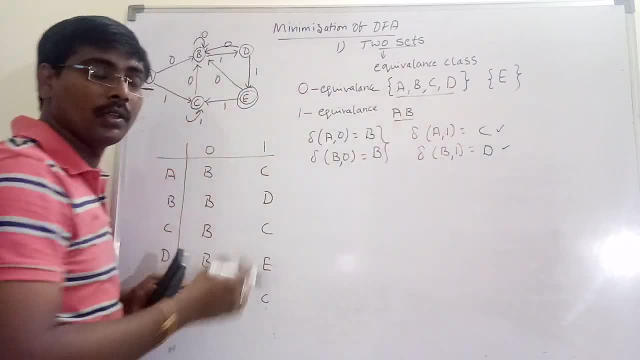 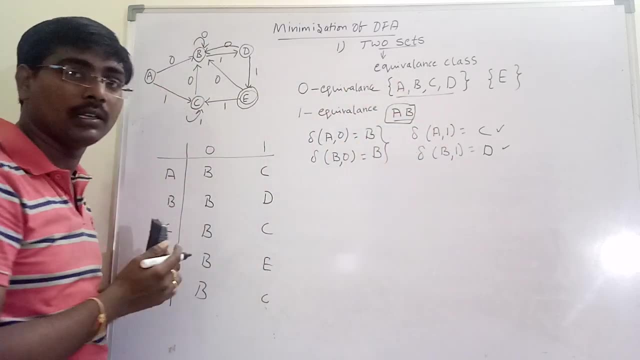 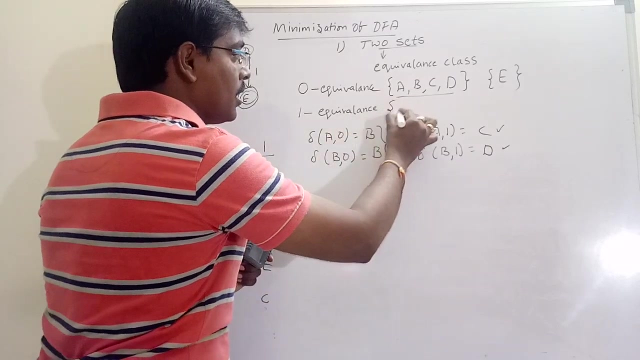 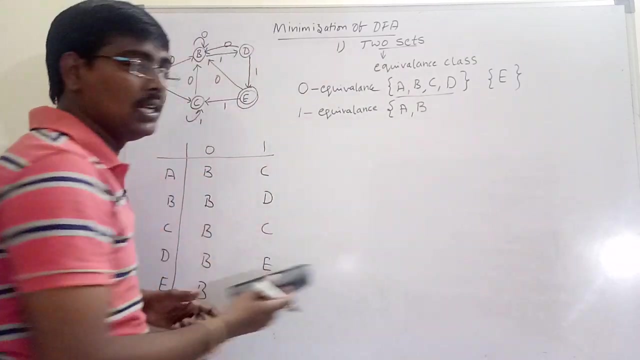 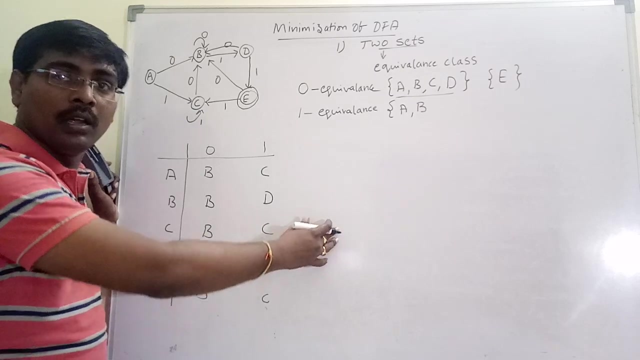 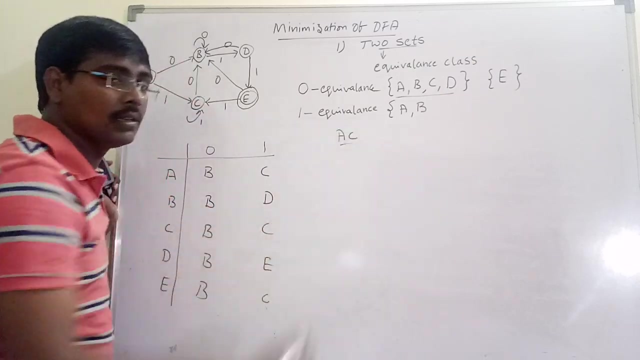 Both C and D belongs to same sex. here both B belongs to same sex. that means A- B are equivalent. A B are equivalent. so I am writing thus: says A B, A B are equivalent. Next I want to check C. so C is equivalent to either A or B. because A and B are equivalent. now I am comparing C with either A or B. both are same. suppose I am comparing A- C. check whether the two states A and C, are equivalent or not. same procedure. 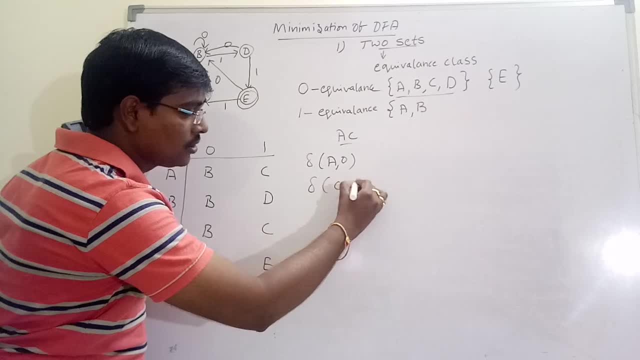 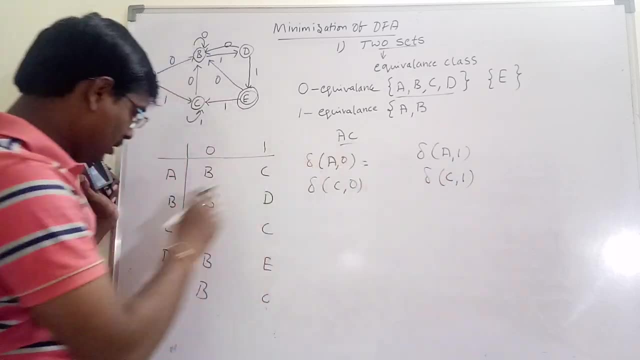 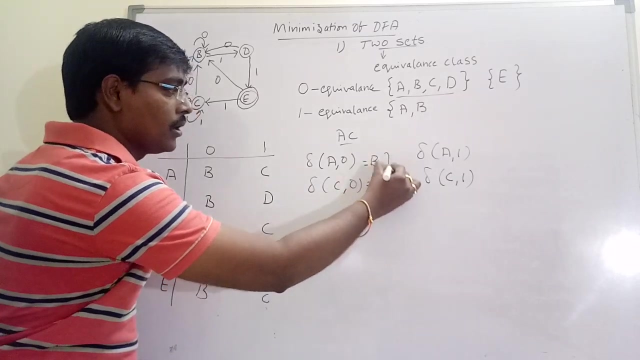 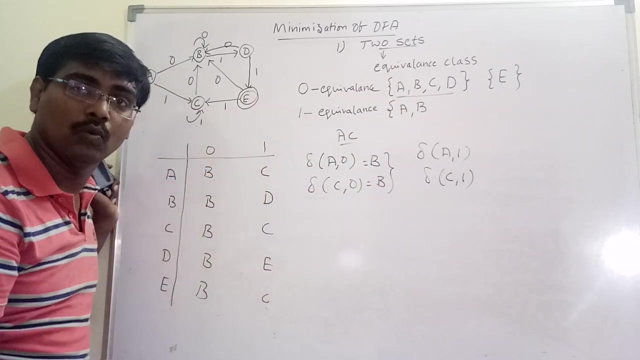 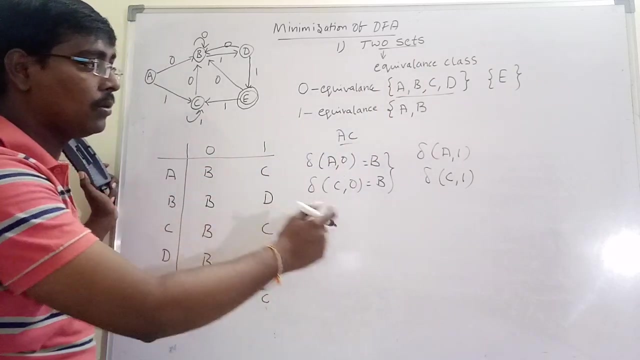 delta of A: 0, delta of C: 0, delta of A: 1, delta of C: 0.. So delta of A: 0 moves to state B. delta of C: 0 moves to state B, so B. we have to check in 0 equivalence class only. we are constructing 1 equivalence class, so we have to check in 0 equivalence class. B belongs to same sex, so no problem. 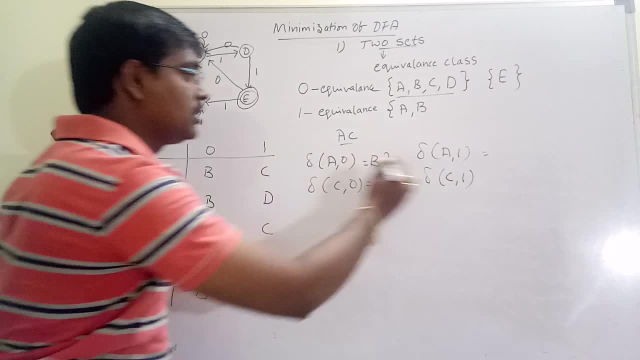 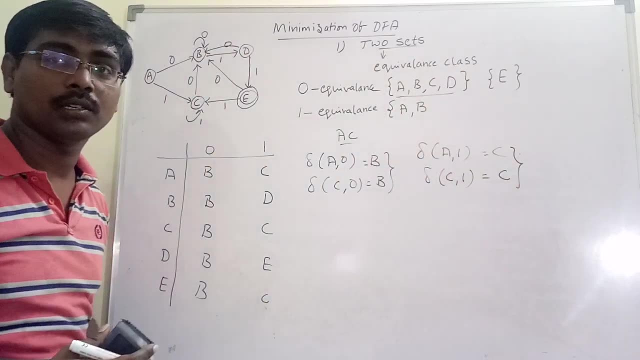 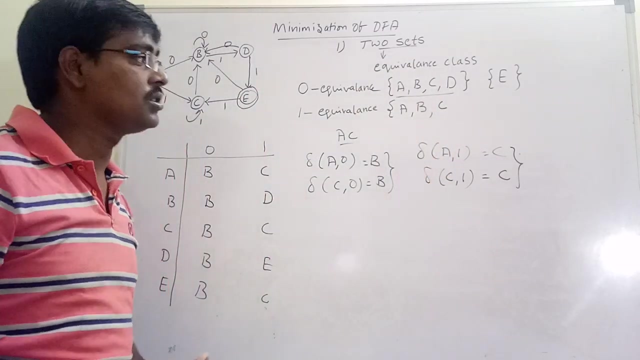 delta of A: 1 value is C. delta of C: 1, the value is B is also C. The C belongs to same set. C also belongs to same set. That means A, B, C, all belongs to same set. That means A and B are equivalent. A and C are equivalent At the 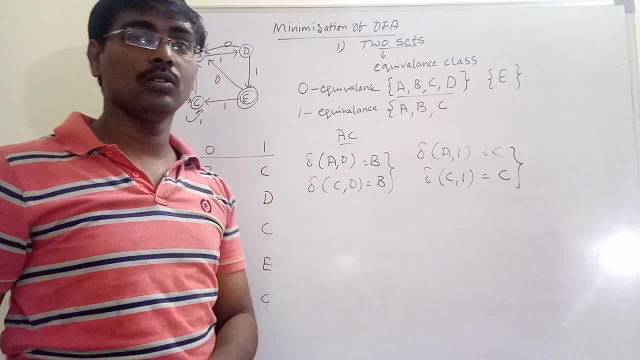 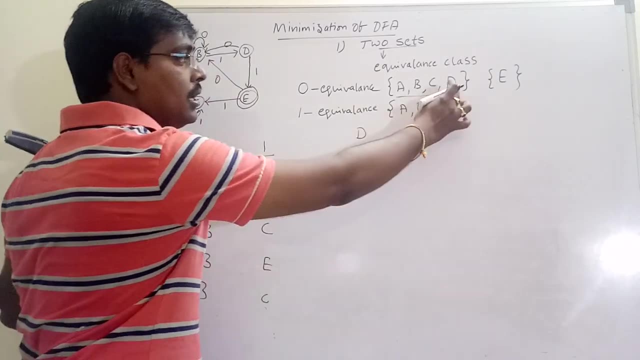 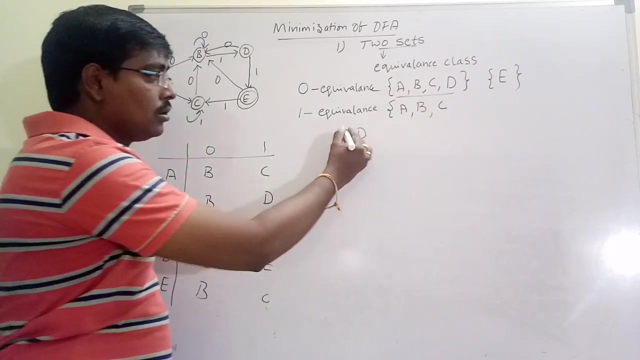 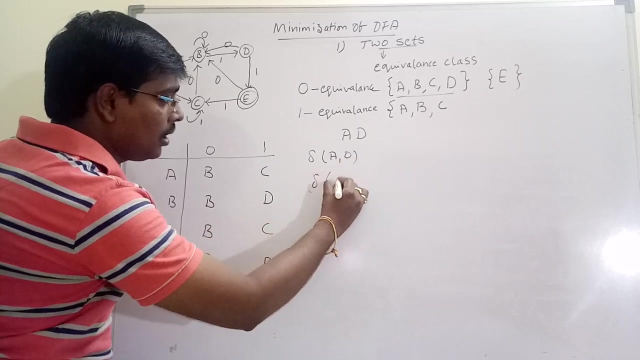 same time. if A and B are equivalent, that means B and C are also equivalent. Next compare D. Check equivalent of D. We have to check equivalent of D with either A or B or C, because all these three are equivalent. So suppose I am checking A D Delta of A. 0.. Delta of. 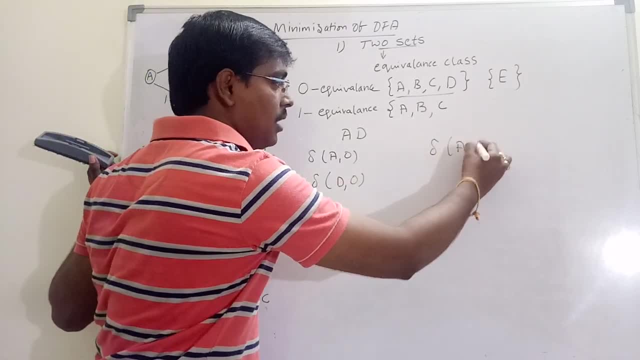 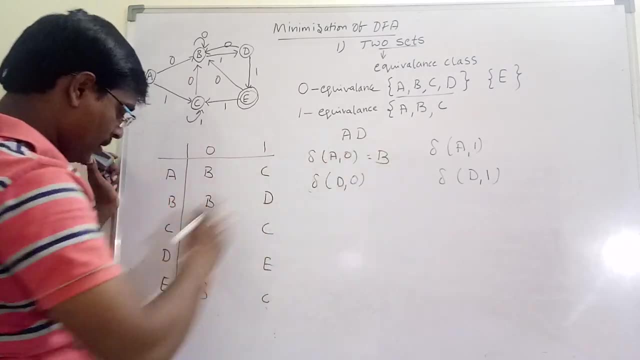 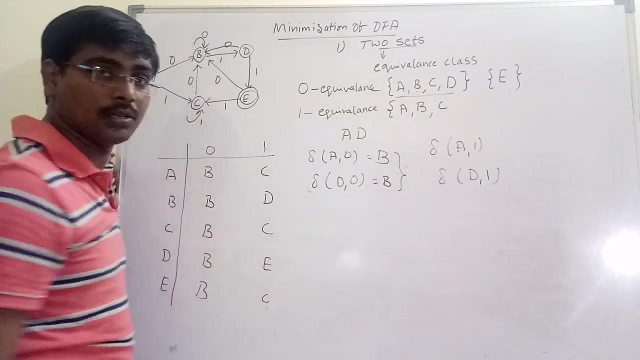 D: 0.. Delta of A: 1. Delta of D: 1. Suppose: delta of A: 0 value is B. D: 0 value is B. So on input 0, both belongs to same set. Now check on input 1.. Delta of A: 1 is C. 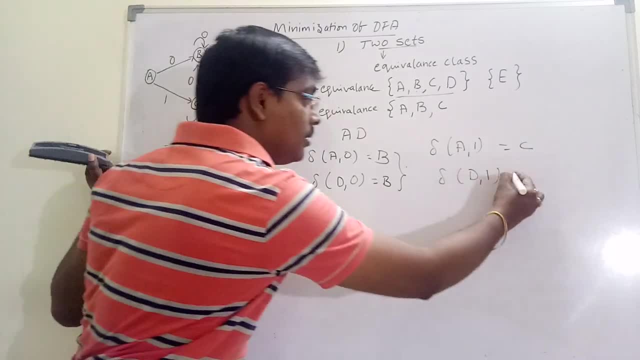 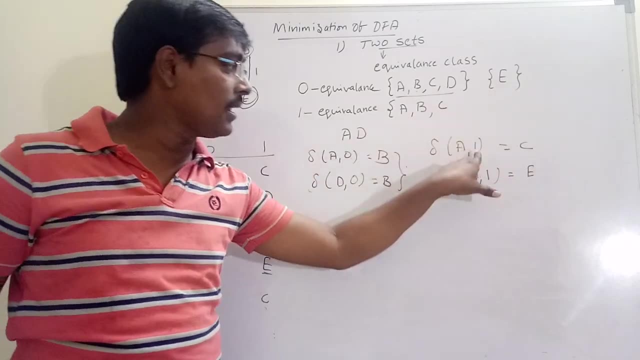 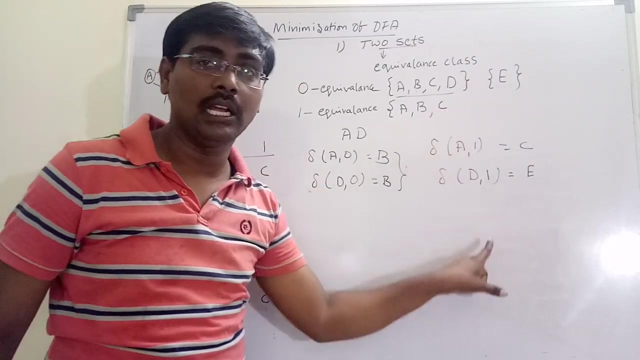 Delta of D: 1 is E. Check. C belongs to set 1.. E belongs to some other set. On transition 1, these two moves to different sets. That means A and D are not equivalent. That means all these three are equivalent. So on input 1, both belong to same set. Now check on. 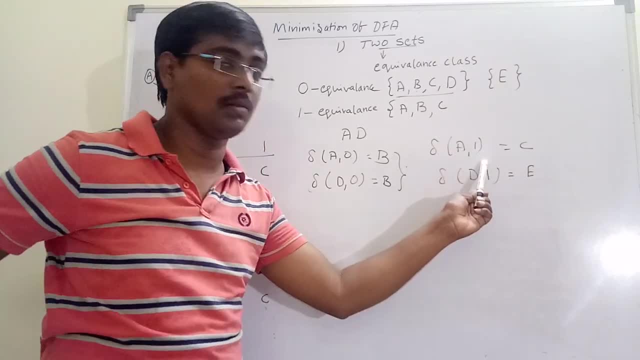 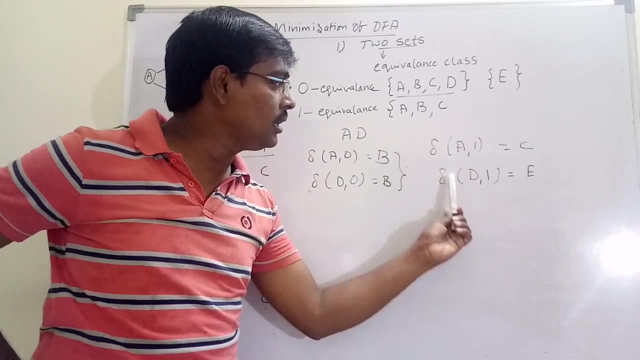 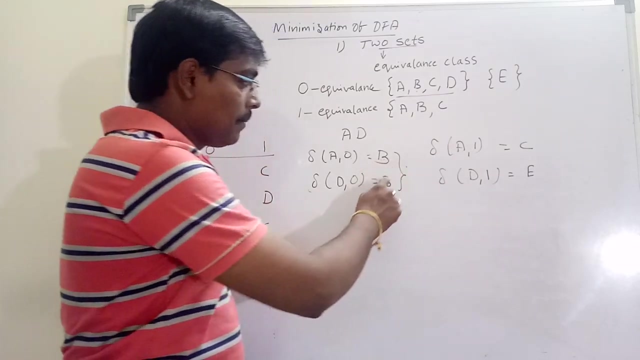 input. 2. After performing transition on a particular input symbol: performing transition on a particular input symbol: on that symbol, if both the states moves to a state within the same set, then those two are equivalent In this here, B and B on input symbol there. 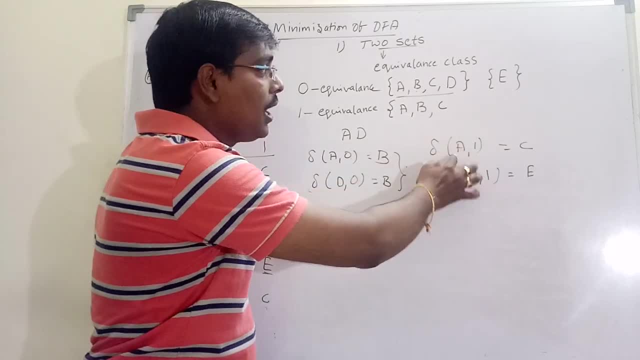 is no problem On input symbol 1,. A moves to this set, That is, on input A on 1,. we are moving to this set For D on input 1,. we are moving to this set For D on input. 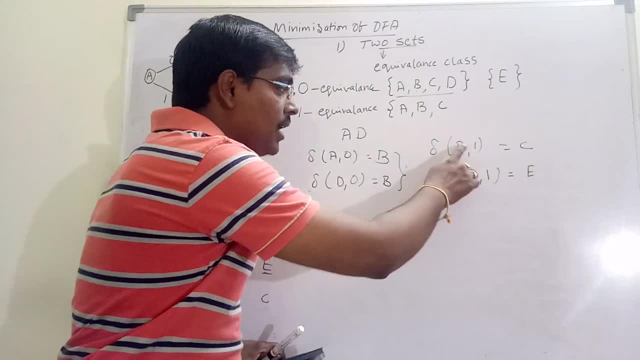 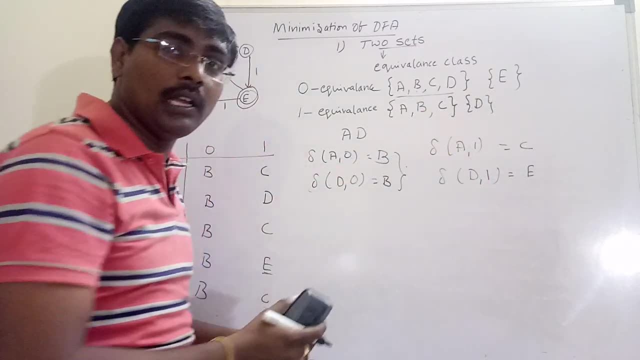 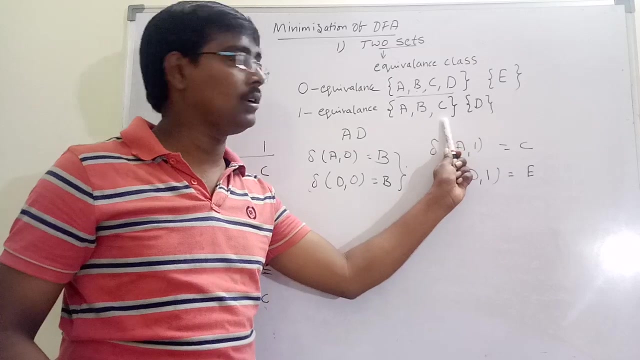 1, we are moving to some other set. That means A and D are not equivalent. So divide A and D are not equivalent means obviously B and D also not equivalent. C and D not equivalent because A, B, C are equivalent. So divide D into a separate set And next E. It contains 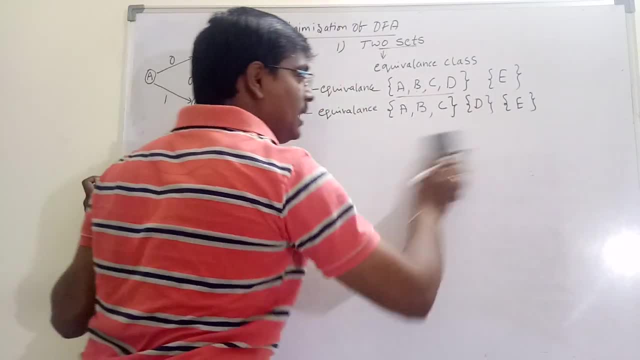 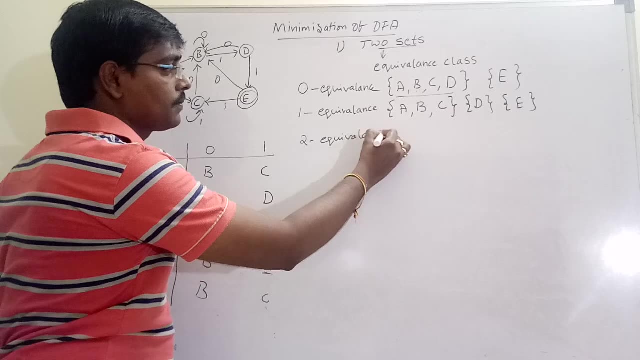 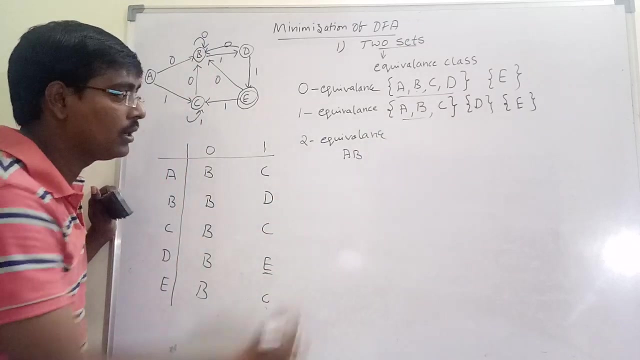 only one thing, No problem. So one equivalence class is completed. Next to our aim is A and B: to calculate two equivalence class. So repeat the same procedure. First, check the set A- B. Check whether A, B are equivalent or not. Delta of A: 0.. Delta of B: 0. Delta. 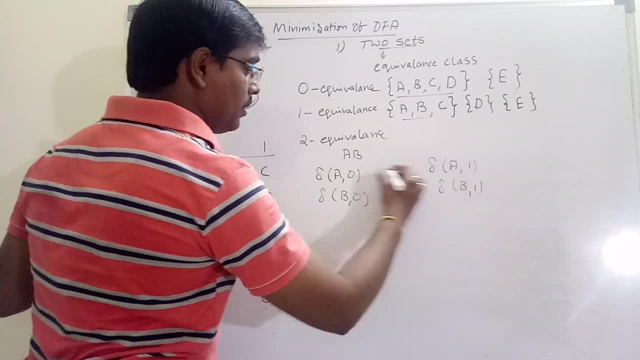 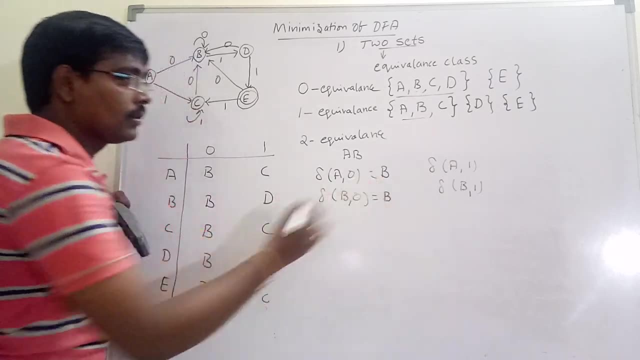 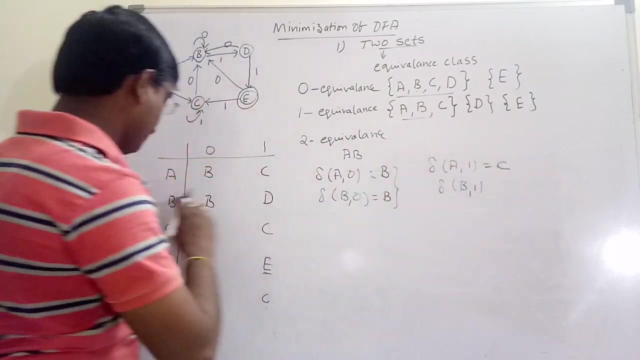 of A: 1.. Delta of B: 1. So A 0 value is B. B 0 value is also B, So both Bs belong to same set. And A 1 value is equal to C. B 1 value is equal to D. A 1 value is equal. 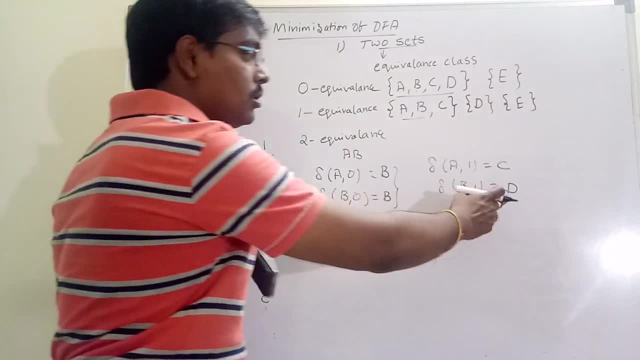 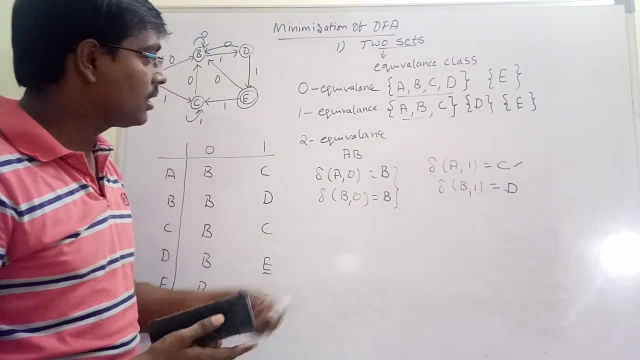 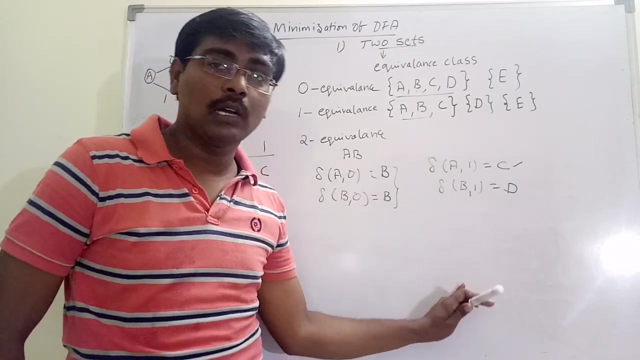 to C. B 1 value is equal to D. C belongs to this set, D belongs to this set. So we are constructing two equivalence class. Then we have to consider one equivalence class only. Suppose we are constructing any equivalence class. We have to consider two equivalence. 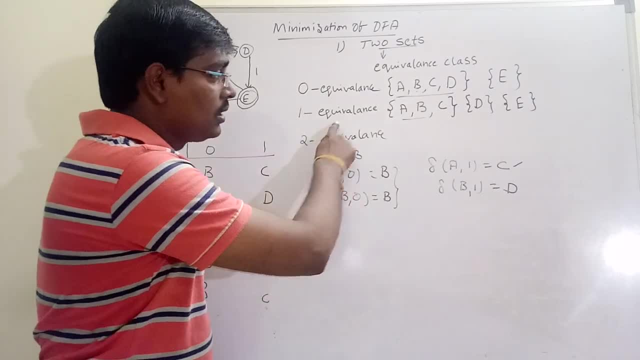 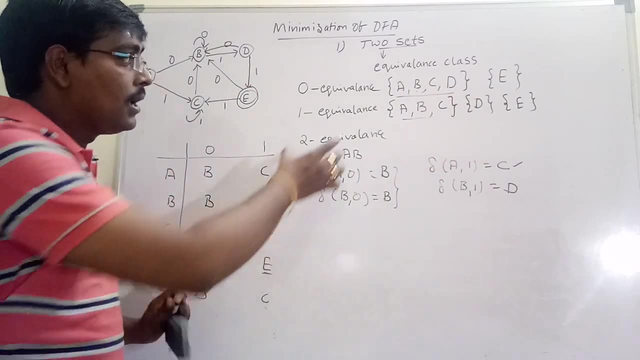 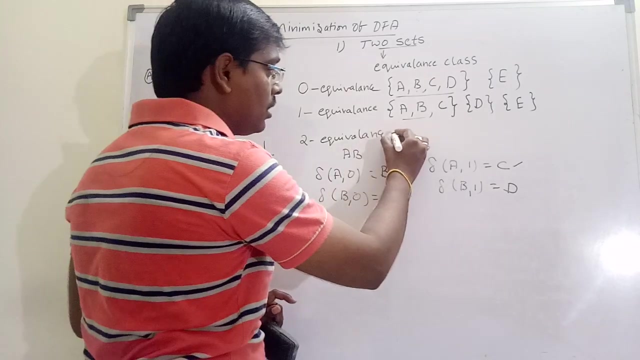 class. So we have to consider n minus 1 equivalence class. So in one equivalence class, A on 1 moves to this set, B on 1 moves to this set. That means, according to this one, A and B are not equivalent. A and B are not equivalent. So A- B. Now we have to check. 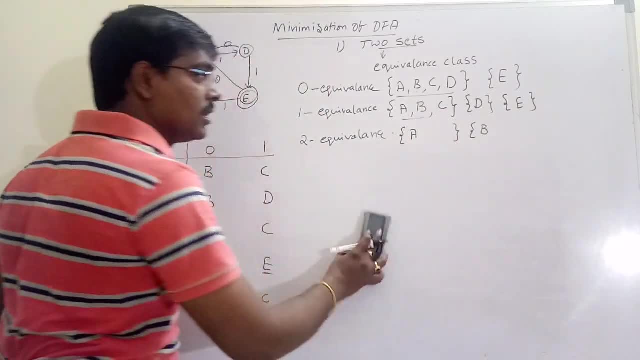 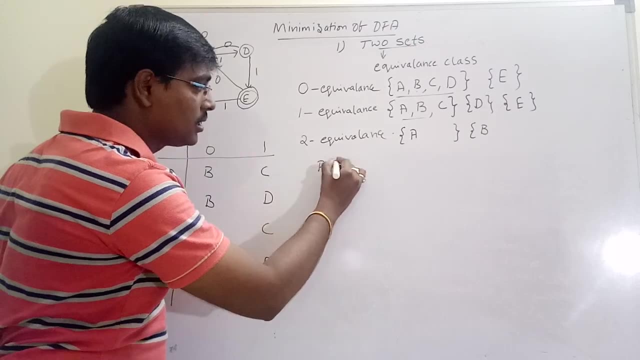 C case. Now we have to check C case. So C is equivalent to D. Now we have to check C case. So C is equivalent to A or C is equivalent to B. We have to check the cases A- C Now. 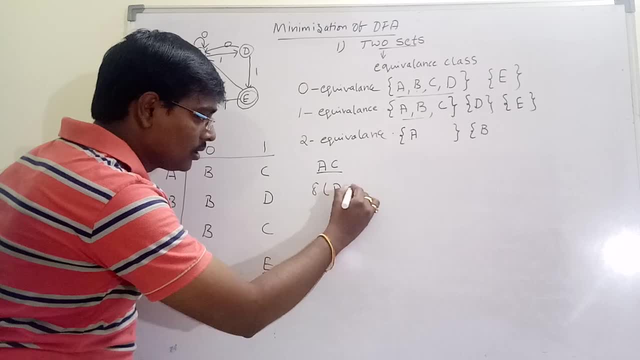 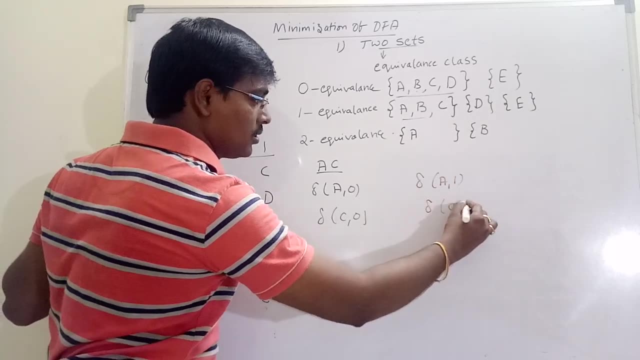 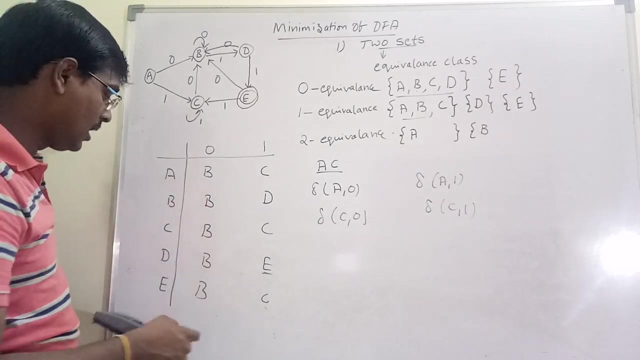 I am checking the case A: C. Delta of A: 0.. Delta of C: 0.. Delta of A: 1. Delta of C: 1.. So Delta of A: 0.. A: 0 value is B, C, 0 value is also B, B, B. So B belongs to. 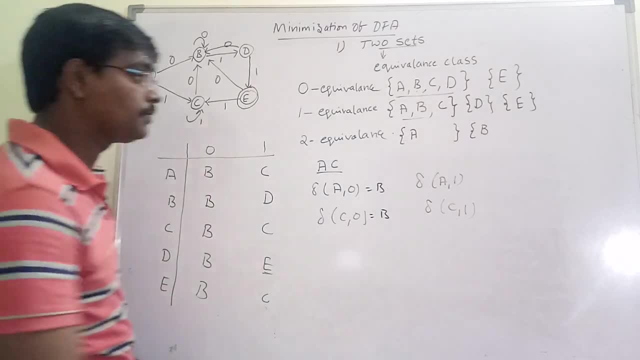 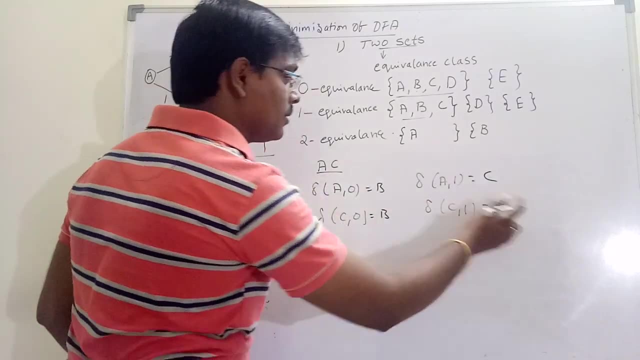 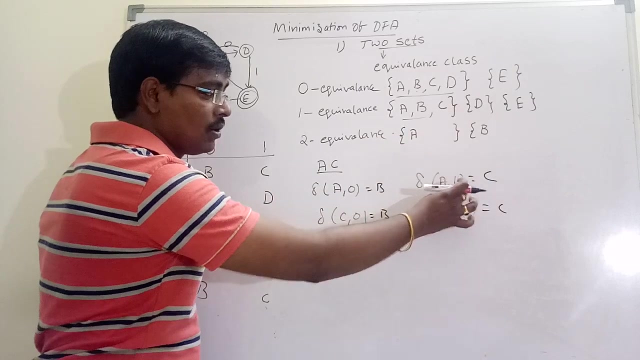 same set. B belongs to same set. Next two: A 1.. A 1 value is C, C 1 value is also C, So both belongs to same set And A 0, B belongs to this set. A 1, C 1, C belongs. 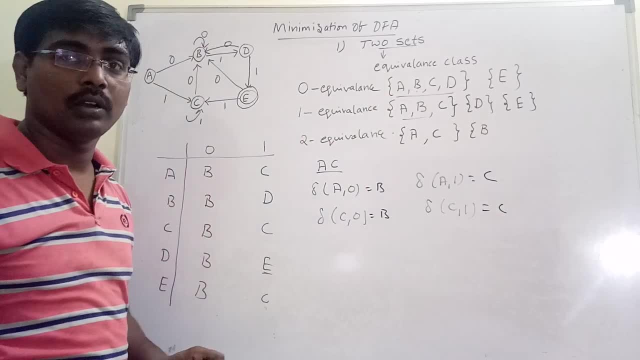 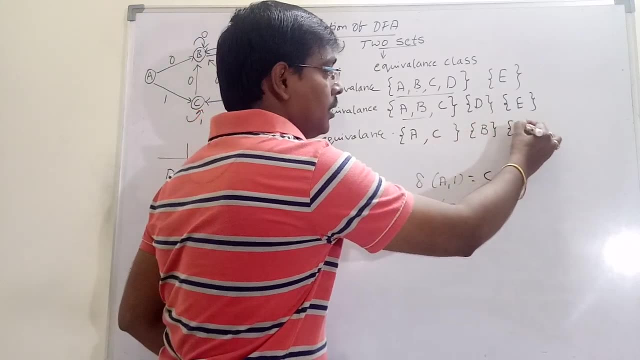 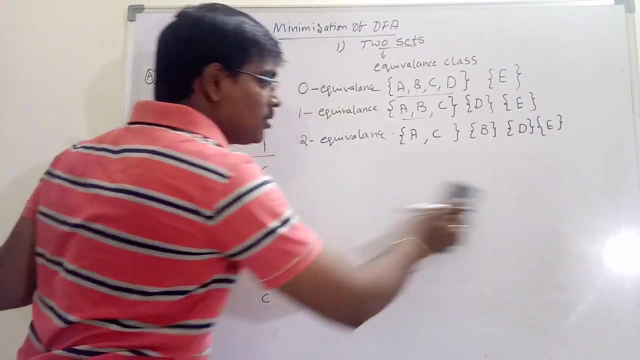 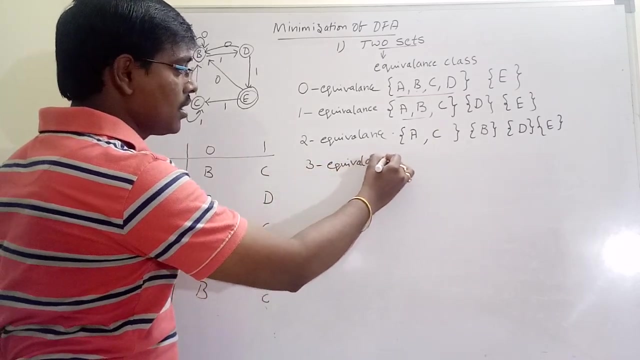 to this set. That means A- C are equivalent classes. A- C are equivalent classes. No need to compare with B. Suppose, if a set contains only single state, That means there is no need to calculate any equivalent class. Next we have to find three equivalence class, Three equivalence: 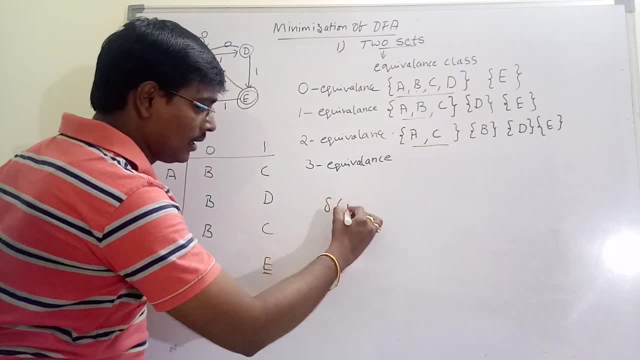 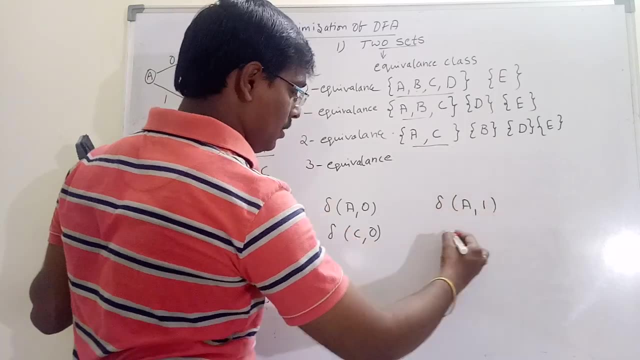 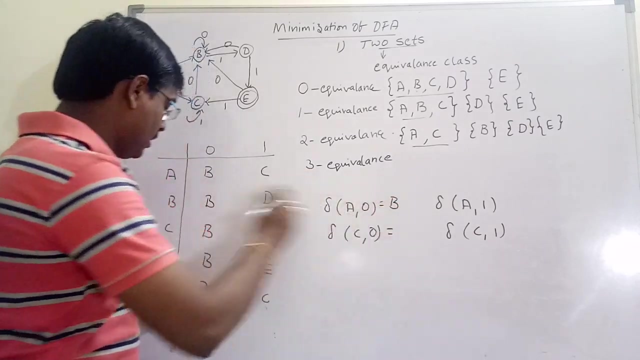 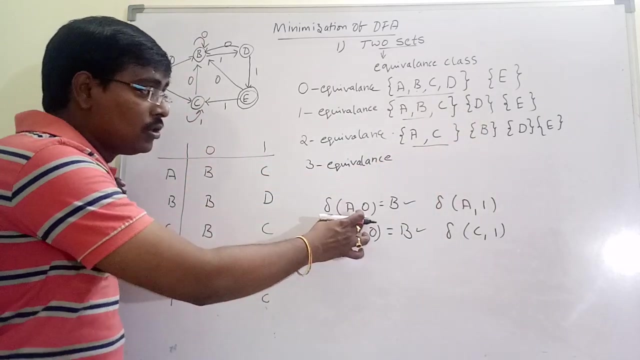 class. We have to compare these two states: Delta of A: 0.. Delta of C: 0.. Delta of A: 1.. Delta of C: 1.. Delta of A: 0.. 0 value is equal to b. delta of c: comma: 0 value is equal to b. both belong to same state. on input: 0. 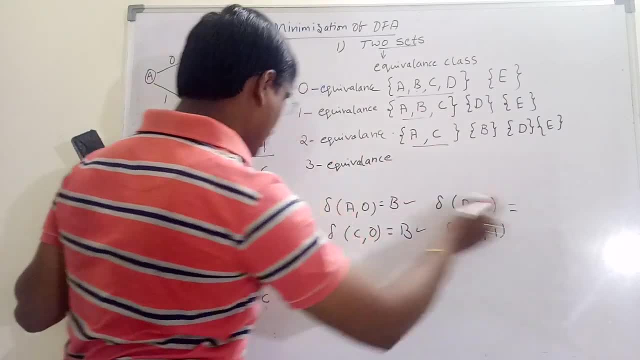 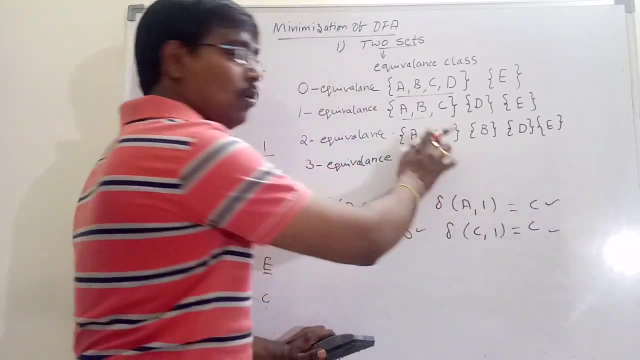 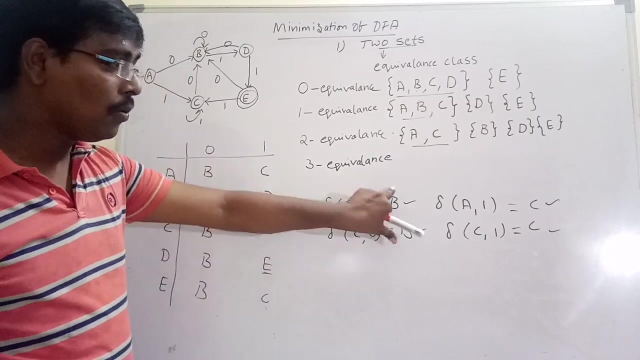 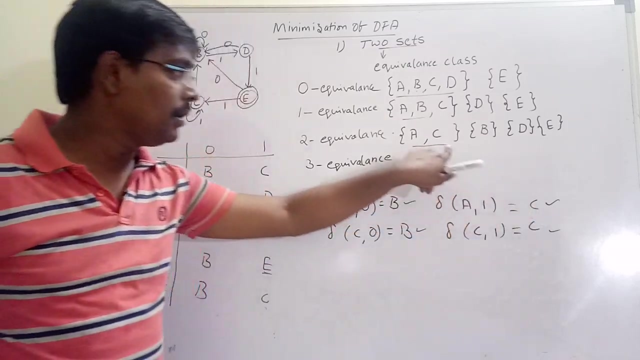 both belongs to same state. a comma 1 value is c. c comma 1 value is also c. on input 1, both belongs to same state. so we have to consider on only one input. on input 0, both belongs to same state, so this to are equivalent. on input 0. on input 1, both are belongs to same. 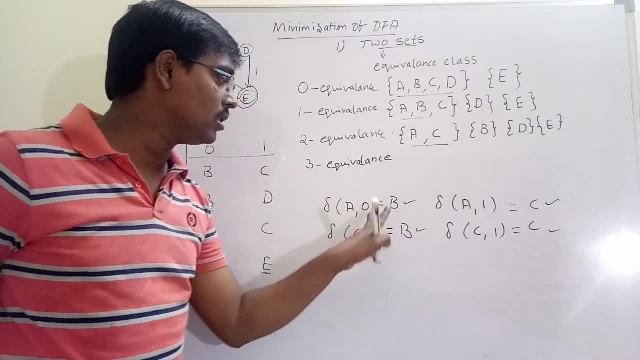 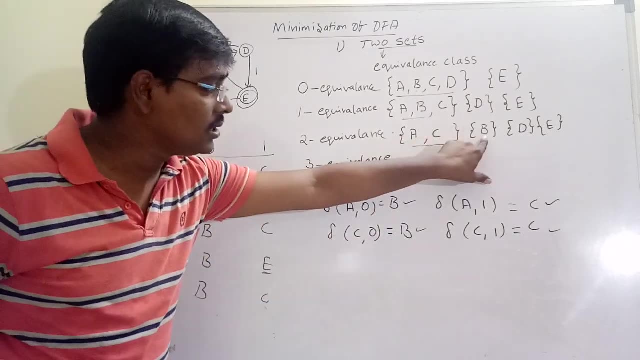 state, that is, these two are equal. at time input 1, that means these two are equal and on input 0 and 1. so if these two all belongs to be, that means this cell, these two are, belongs to some other set if they are not equal, and that is. 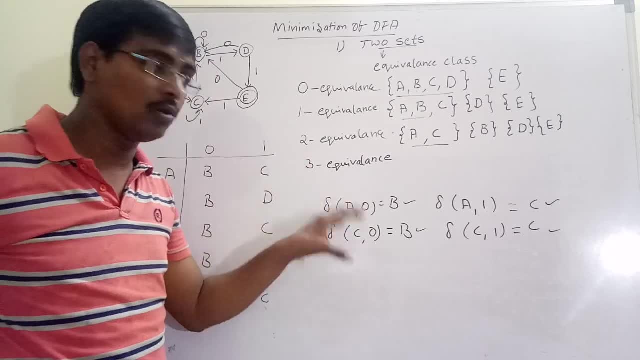 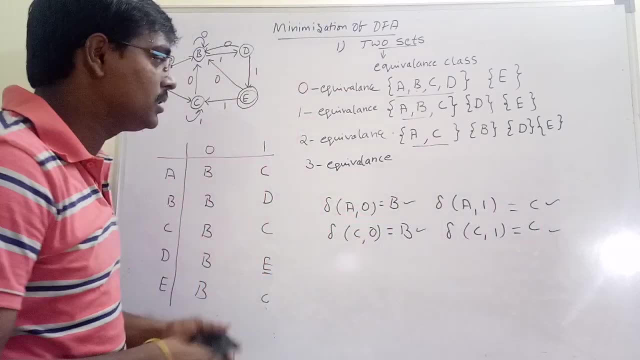 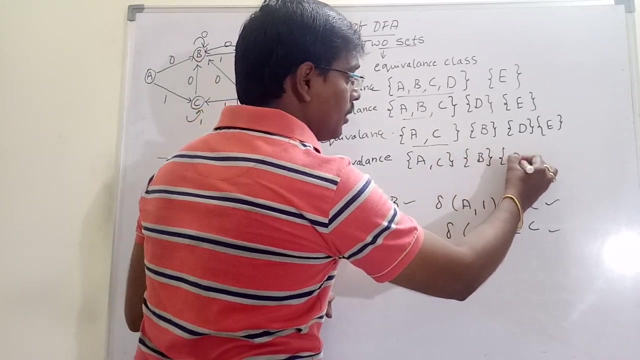 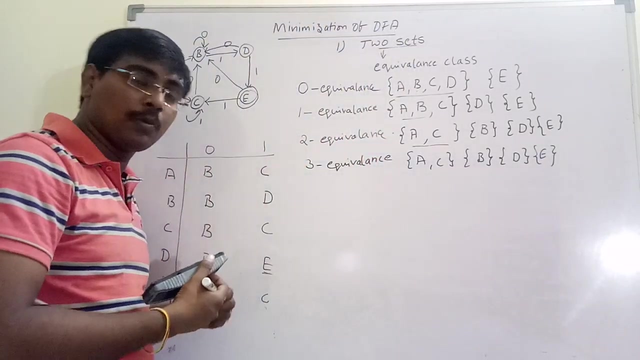 not the case. if these two are on input 0, we have to check on input by import. so input 0, these two are equal, and input 1, this ổi equivalent. that means, finally, a and C are equivalent. we are getting B, D, E. we stop the procedure. so when do we stop the procedure? so at the process of. 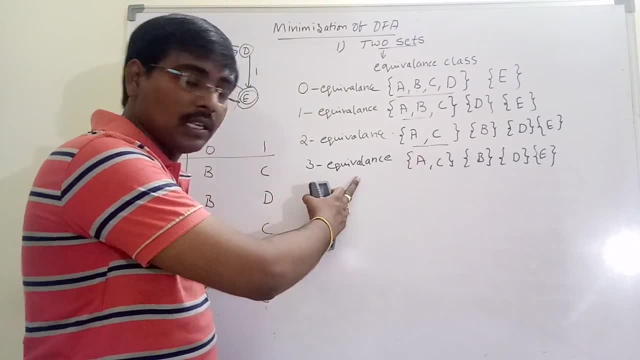 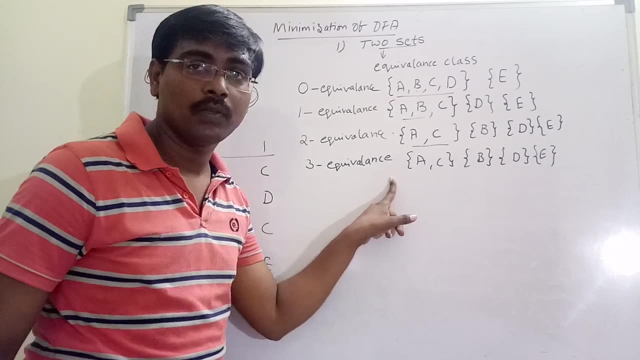 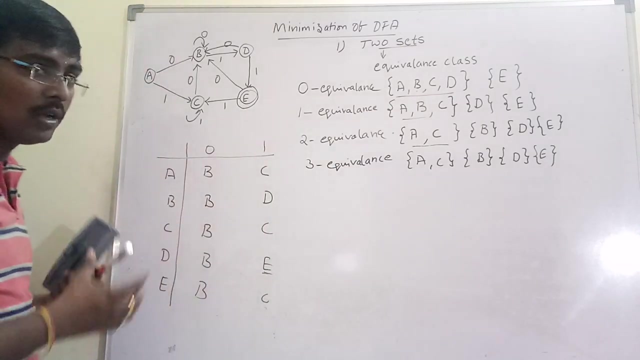 minimization whenever we are getting an equivalence class, that is, we are getting a repeated equivalence class. observe second equivalence class and third equivalence class is same. that means thing next: there is no minimization, so we have to stop the procedure. after completion of this, we how construct? 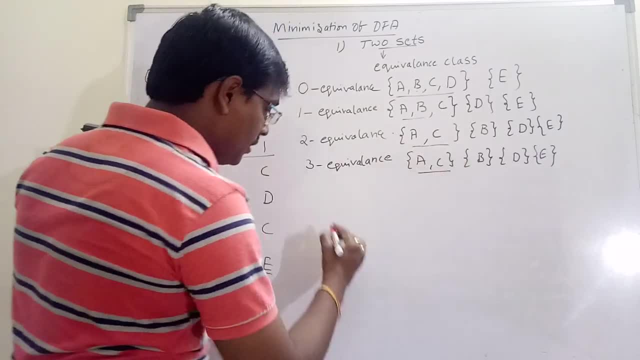 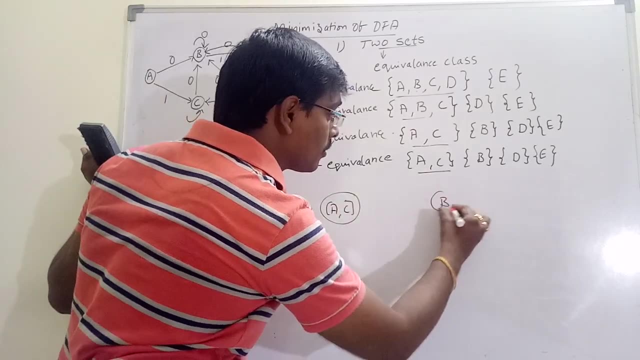 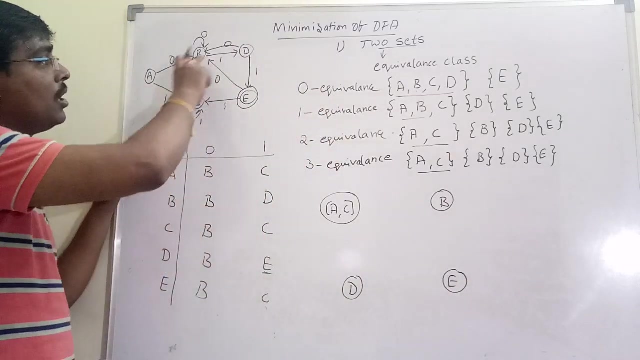 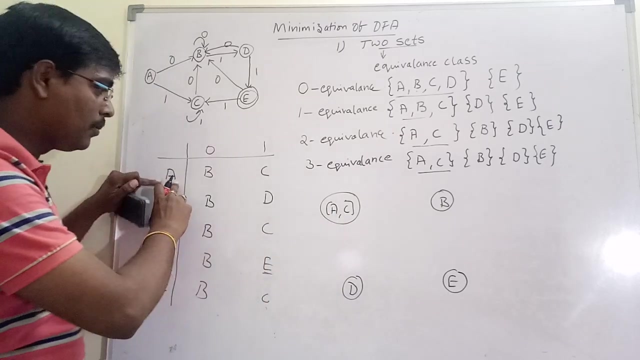 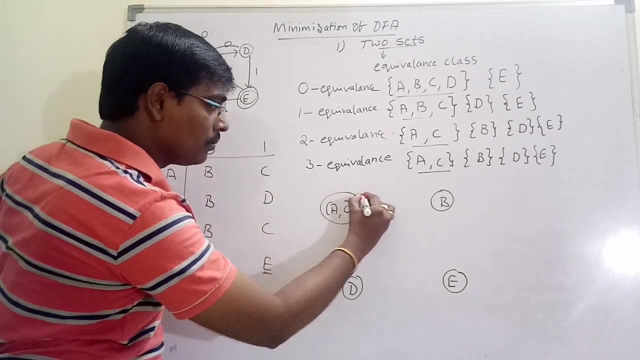 minimized DFA. so this is one state. suppose the states aAC, b, some D, E, now we have four states. previously we have five number of states: after minimization we have five states. so check on a comma, C, suppose on input A. sorry, on state A, with input 0, we are moving to B. similarly, C on input 0, also we are moving to B. that 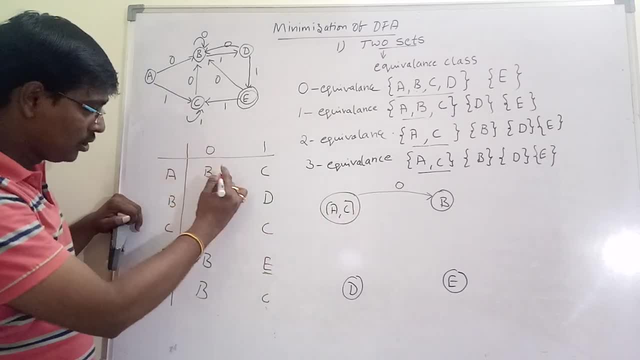 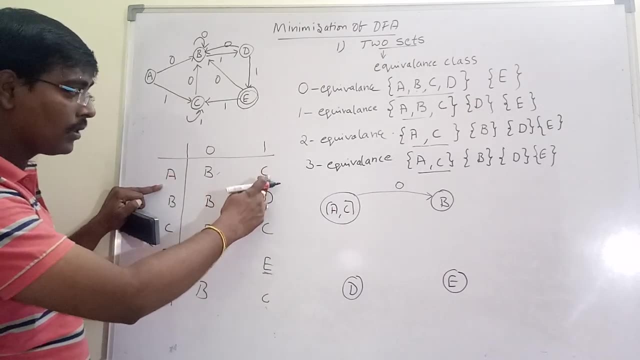 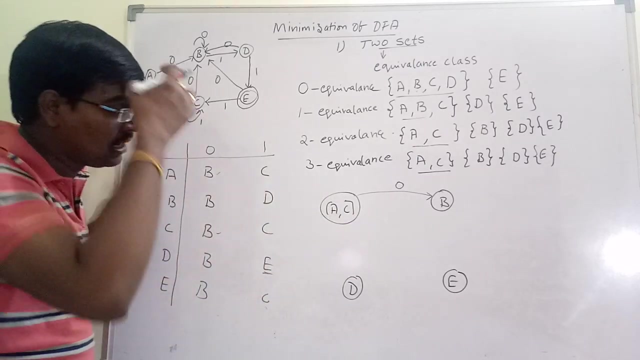 means for the state A comma C. on input 0, we are moving to B next to A. on input 1, we are moving to C. C on input 1 also we are moving to C. that is, these two are equivalent. clearly we are observing on the same input, A comma C on 0. A on 0.